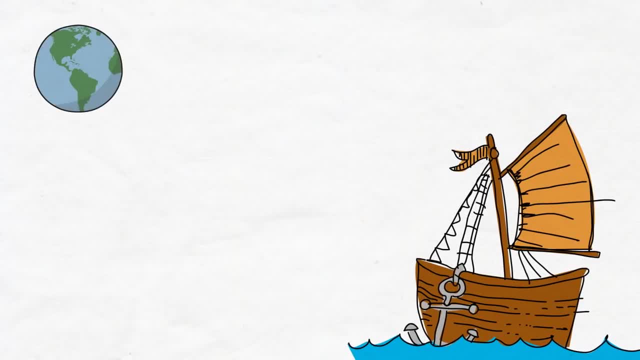 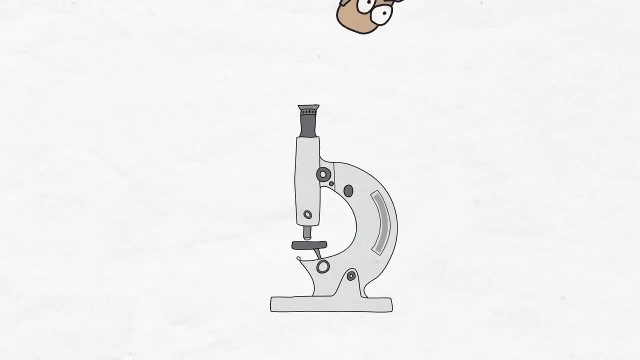 voyage aboard the ship HMS Beagle. The Beagle visited the coasts and islands of South America and Australia, where Darwin observed and collected a wide range of weird and wonderful plants and animals. When he got back to England, he analysed his collection closely. That was. 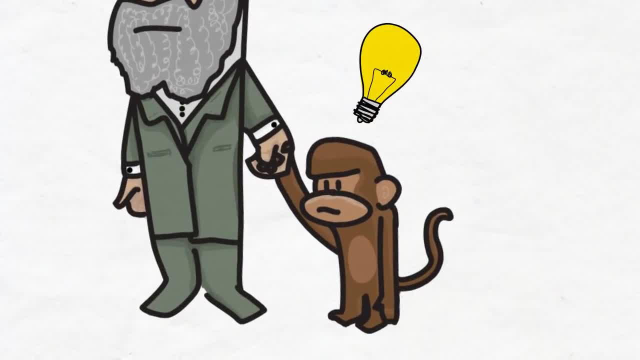 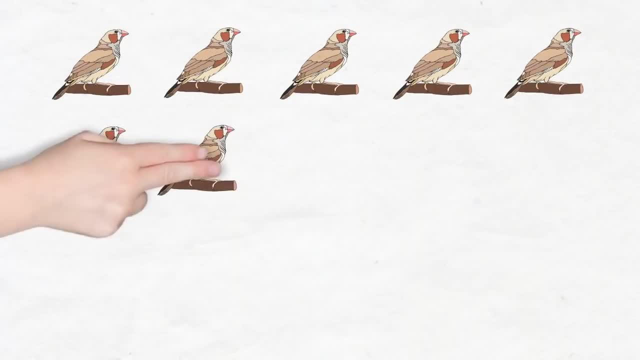 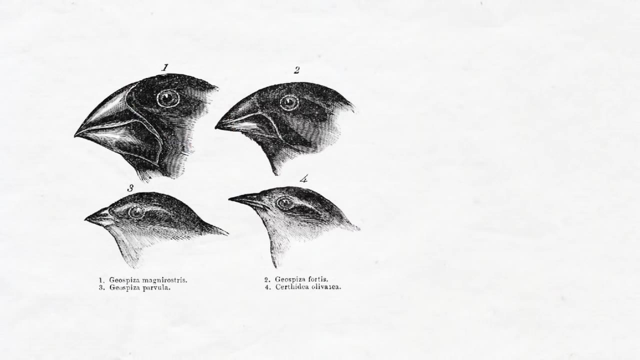 when his ideas about evolution started to form, Darwin had found around 15 different species of finch. when he was on the Galapagos Peninsula, He noticed that the birds were similar to other finches in lots of ways, but their beaks were all different shapes. Darwin looked into it further. He realised that the different 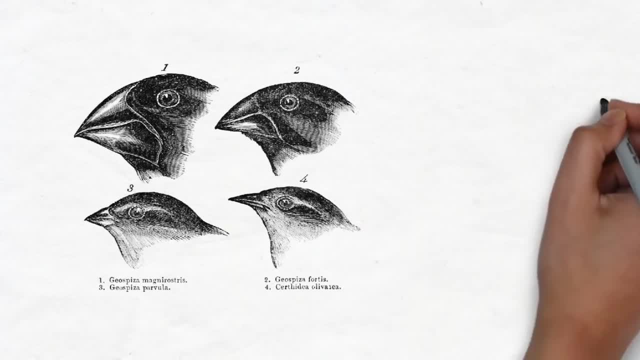 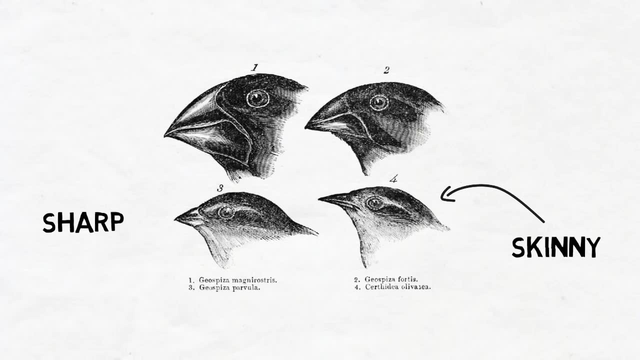 beaks matched the type of food available on each island. The finches who ate insects had skinny pointed beaks so they could pick them up better, and those that ate hard fruits had beaks that were sharp so they could get through the skin. Darwin decided that there. 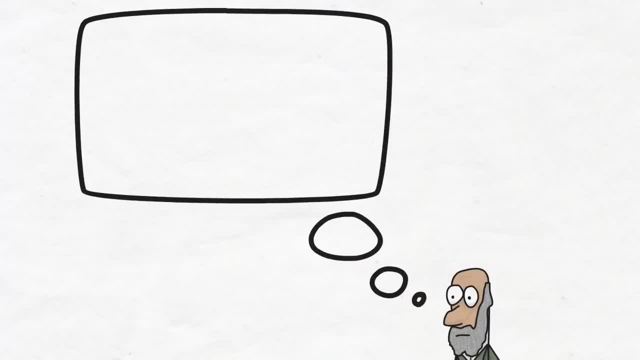 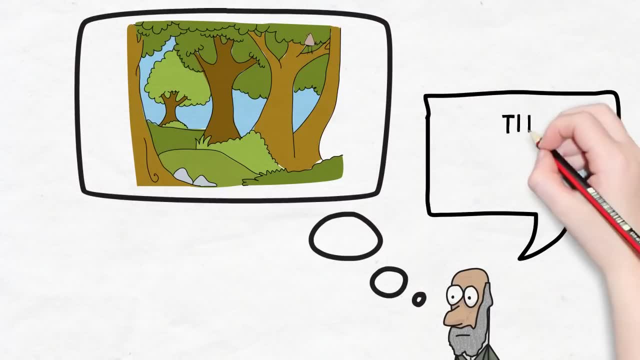 was only one way that the beaks could get through the skin. Darwin decided that there was only one way that this could have happened. The birds must have adapted to their environment over time. This led into another idea, which he called the survival of the fittest. 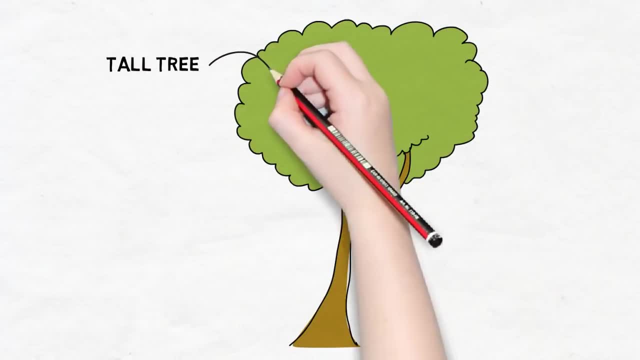 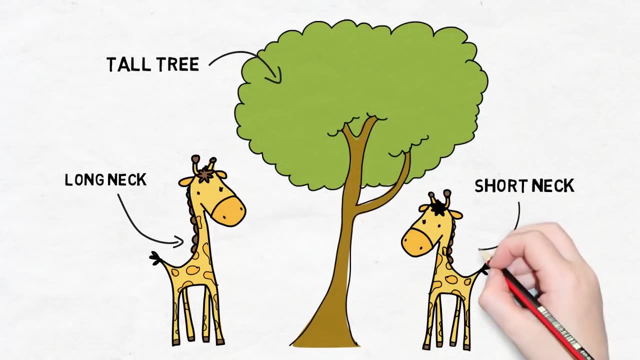 In any environment, plants and animals from the same species show natural variation in their physical characteristics, such as neck length in giraffes. Darwin suggested that those plants and animals best suited to their environment are more likely to survive and pass on their characteristics. 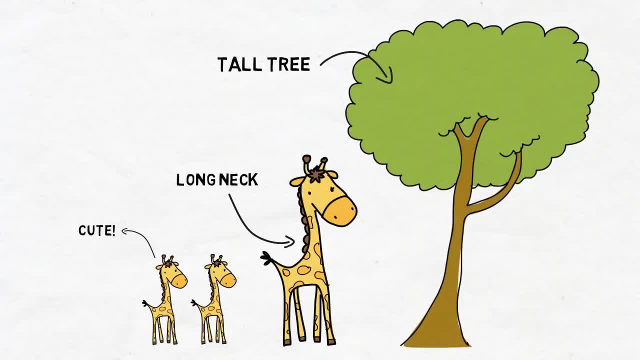 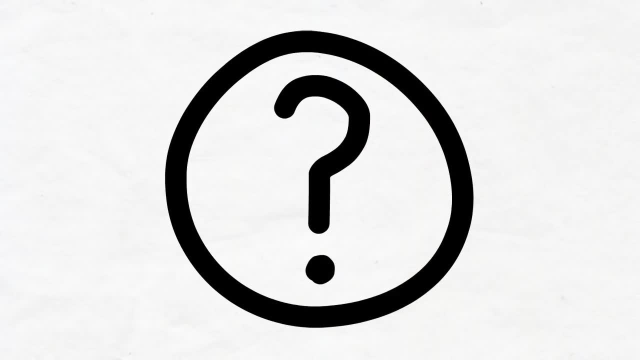 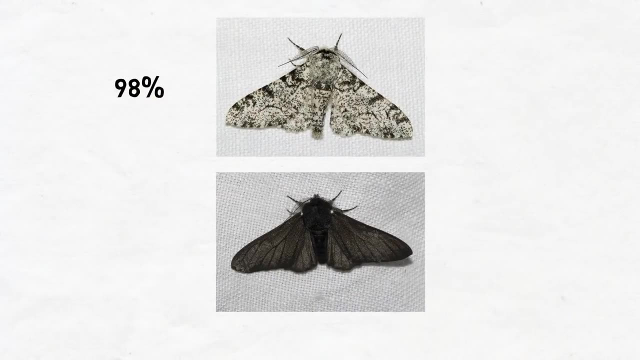 Over a long period of time, the characteristics of the surviving members of the species will come to predominate, Confused. Take the peppered moth. In London in the early 1800s, 98% of peppered moths had light-coloured bodies. Only 2% were dark. The light moths were very 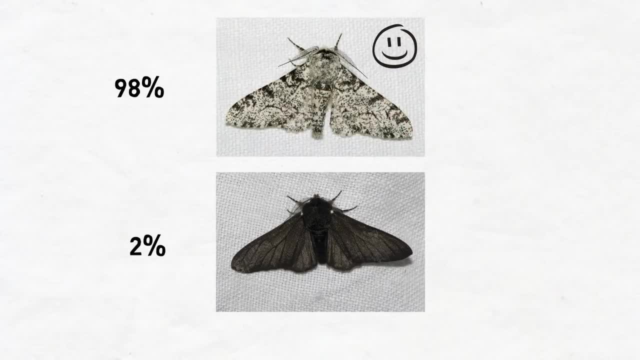 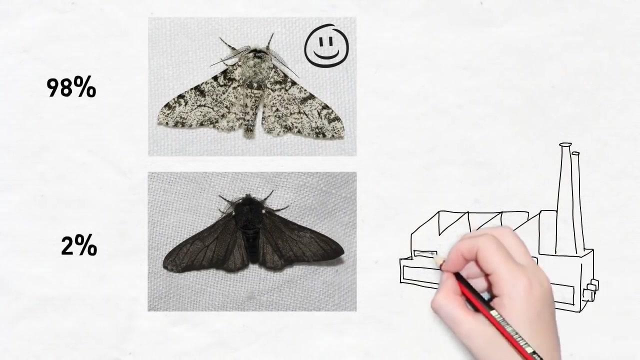 happy because they were the same colour as the trees, which meant that they could easily hide from hungry birds. The dark peppered moths were easy to find and they could easily eat. Then came the factories and the smoke of the industrial revolution. Many trees turned black.